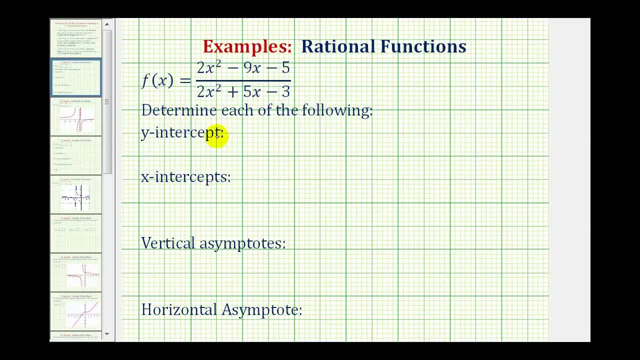 We're given a rational function and asked to determine the y-intercept, x-intercepts, vertical asymptotes and horizontal asymptotes. When working with rational functions, it's often helpful to have the numerator and denominator in factored form. So let's start by factoring both the top and bottom. 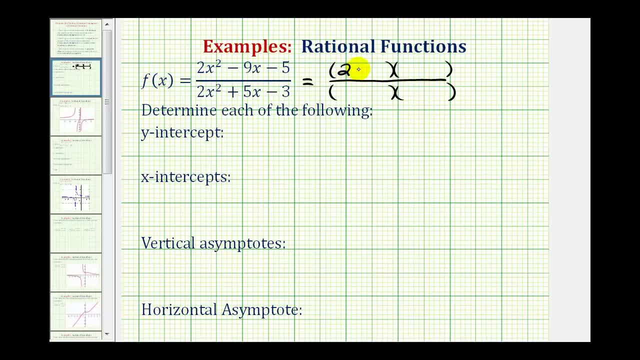 Looking at the numerator, the factors of two x squared are two x and x. The second positions must come from the factors of negative five. The sum of the inner product and outer product is equal to negative nine x. So if we use a factor of negative five here minus five, that would give us negative ten x. 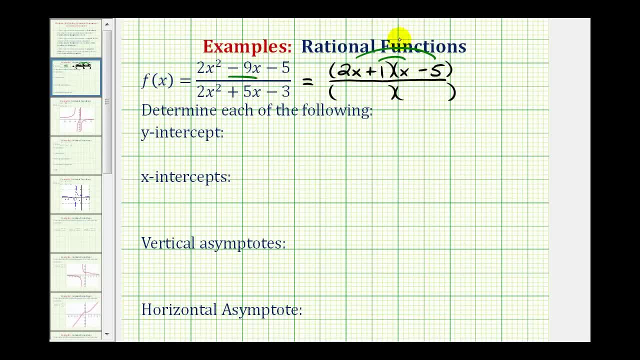 The other factor of negative five is positive one, So negative ten x plus one x is equal to negative nine x, so that's factored correctly. Now for the denominator. we'd have a factor of two x and x here. Now we use the factors of negative three in the second positions. 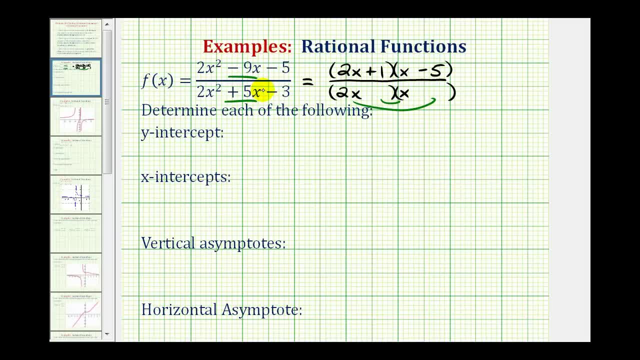 So the sum of the inner and outer product is equal to positive five x. So if we use a factor of positive three here and minus one here, we have positive six x plus negative one. x is equal to five x. Now we'll start by finding the y-intercept. 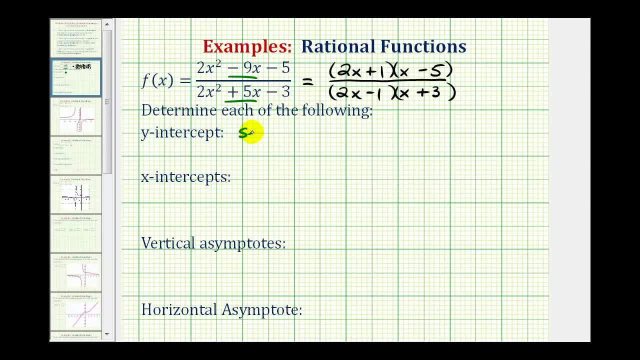 To find the y-intercepts of any function, we set x equal to zero And because this is written in function notation, that means we need to evaluate f of zero. So whether we use the original form or the factored form, it doesn't matter. 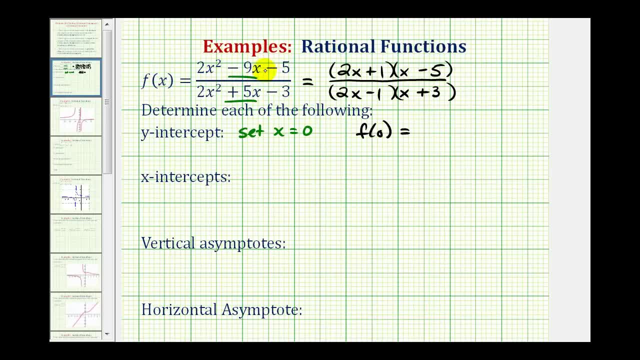 If we use the original form, if x is zero, we would have zero minus zero minus five or negative five divided by zero plus zero minus three or negative three. This result would be the same if we use the factored form as well. This simplifies to positive five-thirds, which means our y-intercept is the point, with an x-coordinate of zero and a y-coordinate of positive five-thirds. 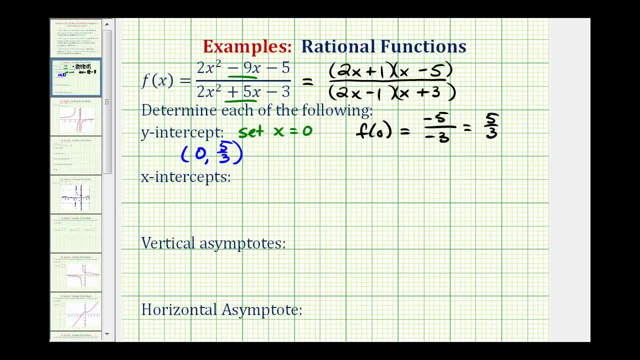 To find the x-intercepts of a function. we set y equal to zero or the function value equal to zero. But because we have a rational function, as long as there aren't any common factors between the numerator and denominator, this function will only equal zero when the numerator is equal to zero. 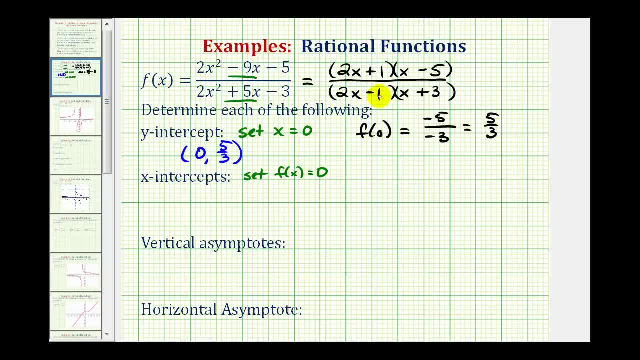 To show why this is true, we'll set f of x equal to zero and then solve for x, So we would have zero equals, in factored form, the quantity two x plus one times the quantity x minus five. all over the quantity two x minus one times the quantity x plus three. 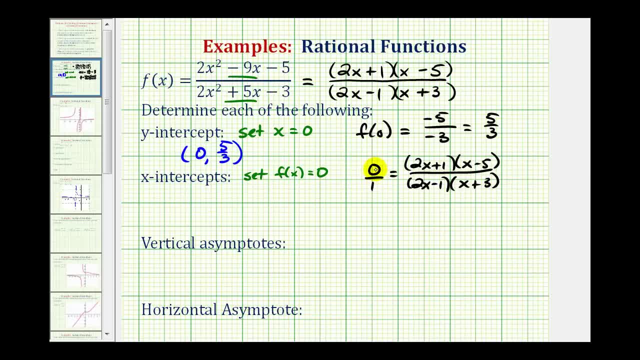 So because this is a fraction, if we put zero over one it's still equal to zero. and now we can solve by cross-multiplying. But notice, when we cross-multiply we would have: one times the numerator is equal to zero times the denominator. 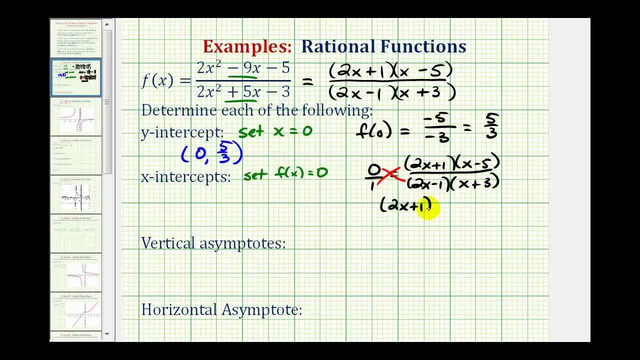 which would just give us the equation: the numerator equals zero. So as long as there aren't any common factors between the numerator and denominator, the x-intercepts can be found by setting the numerator equal to zero. Two x plus one is equal to zero when x equals negative one-half. 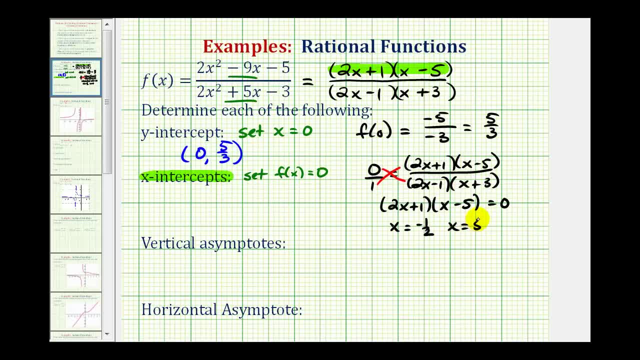 and x minus five is equal to zero when x equals five. So we have two x-intercepts. They're the points negative, one-half comma zero and five zero. Now to determine the vertical asymptotes of a rational function. again, as long as there aren't any common factors between the numerator and denominator. 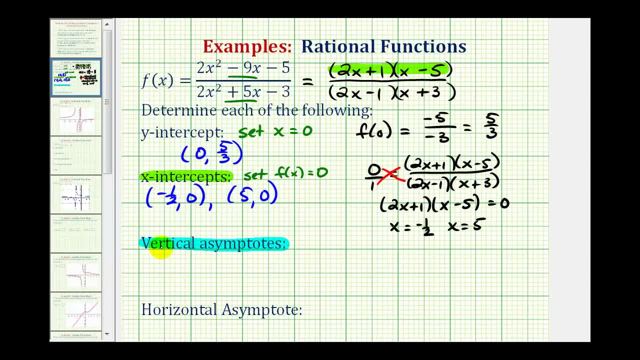 the values of x that make the denominator equal to zero. give us the equations of the vertical asymptotes. So we can find the vertical asymptotes by setting the quantity two x minus one times the quantity x plus three, equal to zero If there are common factors between the numerator and denominator. 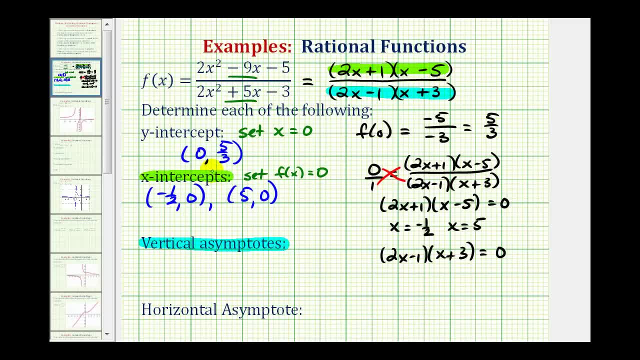 the zeros of the common factors give us wholes, not x-intercepts or vertical asymptotes. So two x minus one is equal to zero when x equals positive one-half, and x plus three is equal to zero when x equals negative three. Remember vertical asymptotes are vertical lines. 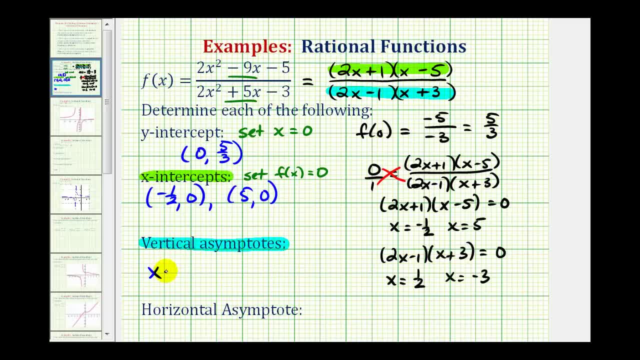 so the equations of the vertical asymptotes are: x equals one-half and x equals negative three. And now for the last question. we're asked to determine the horizontal asymptotes, which is really asking us to determine the end behavior or long-run behavior of a rational function.